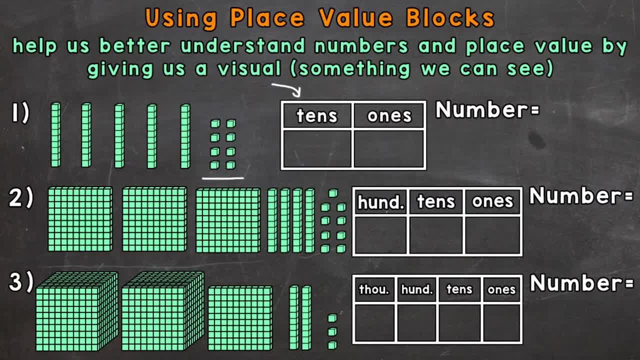 like I just mentioned, and are going to be represented in the ones place. So let's see how many we have. So we have 1,, 2,, 3,, 4,, 5,, 6,, 7, and 8. So we have 8 ones, which has a value of 8.. So 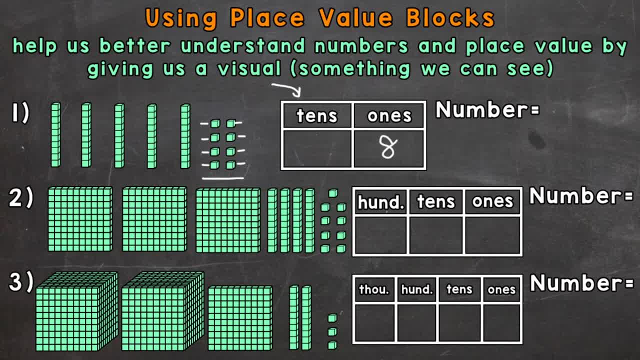 we're going to put an 8 in the ones place, So these blocks right here represent the ones place that are our number. Now the stacks that are over here. there are 10 individual blocks in each stack, So we don't need to count each individual block. We can count the stacks because they are. 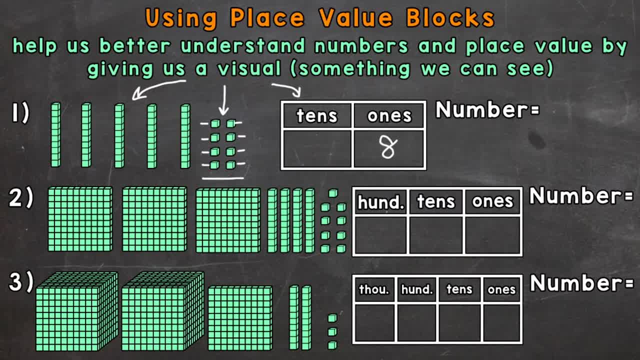 grouped into groups of 10.. So let's see how many stacks we have: 1,, 2,, 3,, 4, and 5.. So we have 5 groups of 10, which has a value of 8.. So we're going to put an 8 in the ones place. So let's see. 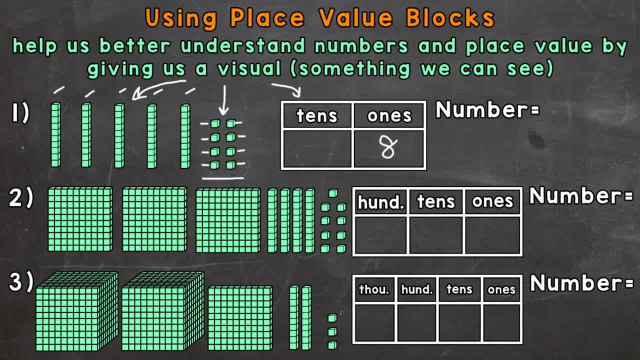 how many stacks we have. So we've got 8 in the ones place. So we're going to put a 5 in the tens place, which again has a value of 50.. 5 groups of 10.. So our number in standard form we would write: 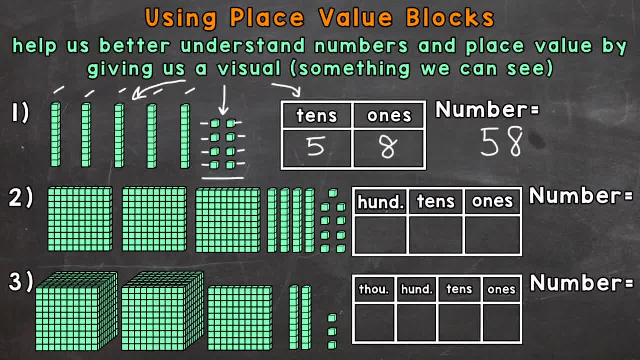 58. And just to recap, the 8 represents 8 wholes or 8 ones, and the 5, because it's in the tens place, represents 5 groups of 10, which has a value of 50.. Let's go to number two here, where we are going to include some different blocks here and actually 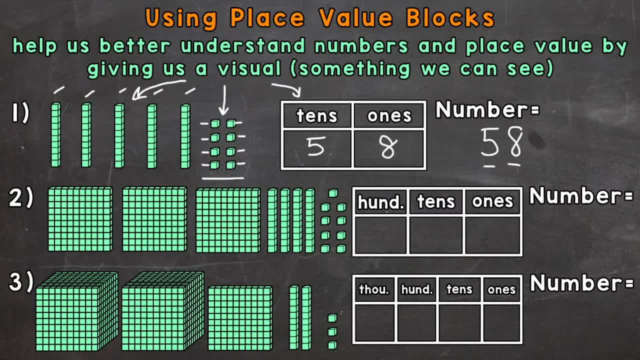 go to a three digit number, So we're going to go to the hundreds place. Let's check our ones first. So right here. So we have one up top, two, three, four, five, six, seven, eight, nine ones. So let's. 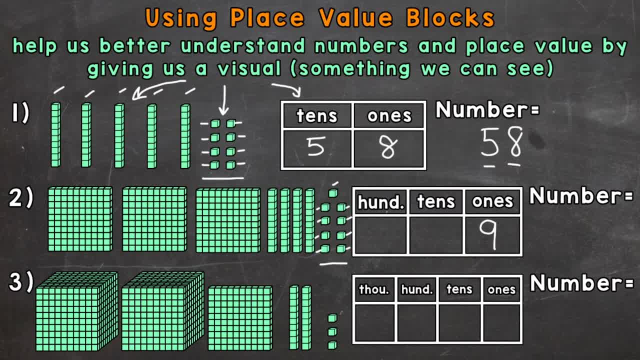 put a nine in the ones place. Let's check our groups of 10.. So the stacks of 10, we have one, two, three and four, So four groups of 10, which has a value of 40. And we represent that by putting. 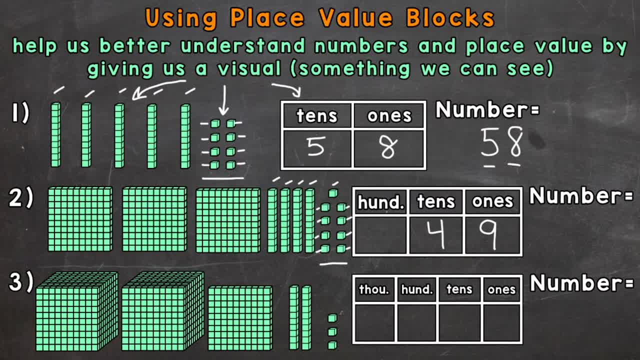 a four in the tens place for groups of 10.. Now, lastly, we have these squares over here. Now, those represent 100, because there are 100.. 100 place value blocks within each of those squares. So let's see how many we have. So we have. 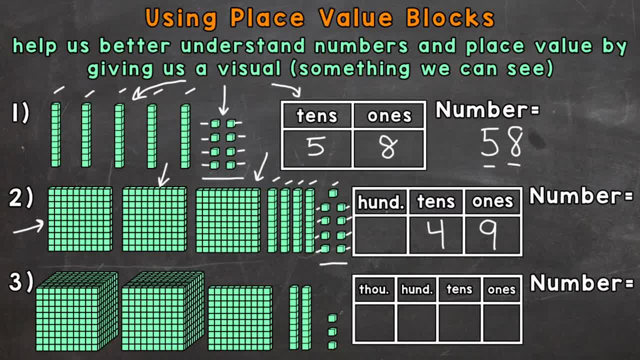 one right here, two and three. So we have three groups of 100, which has a value of 300.. So we represent that by putting a three in the hundreds place right here. So our standard form, or writing the number out as we normally would, would be 349.. So the nine represents nine ones. The four: 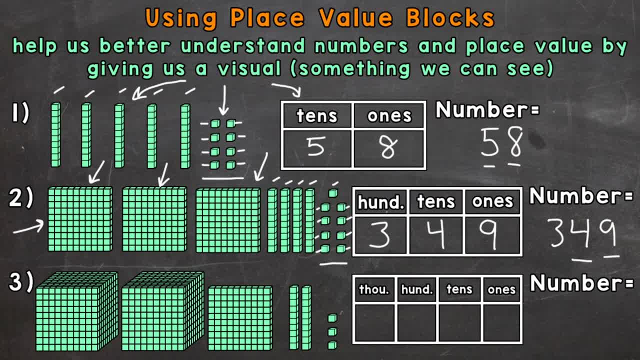 represents four groups of 10,, which has a value of 40. And then we have three groups of 100, which has a value of 300.. And that gives us 349.. So, lastly, number three, we are going to start. 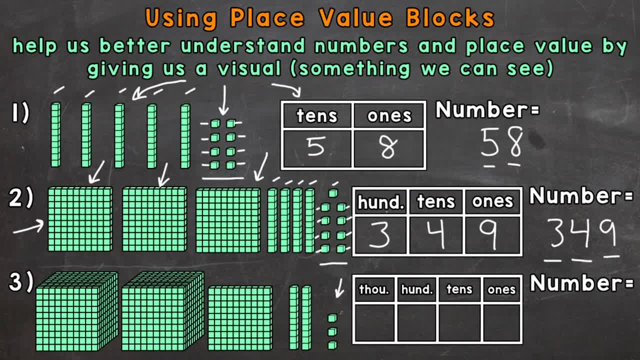 with the one Right here, and we have one, two, three ones. So let's put a three in the ones place. Next, we have one two groups of 10, which has a value of 20. So let's put a two in the tens place. Then for our 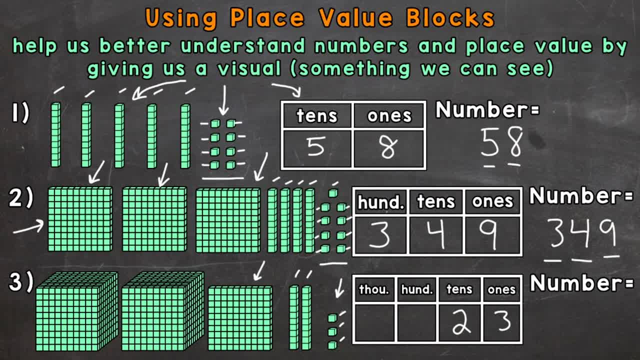 hundreds we have one. So one group of 100 has a value of 100. And we represent that by putting a one in the hundreds place. So let's put a three in the ones place. Next we have one, two groups of. 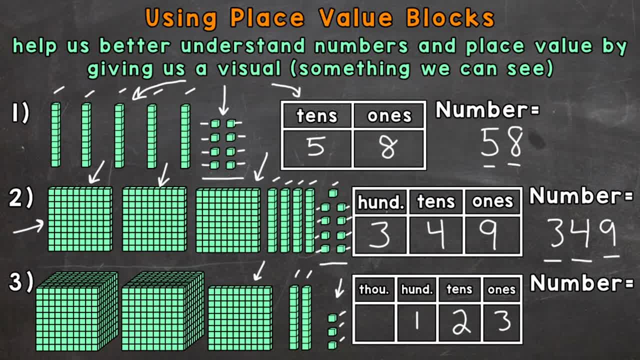 100 in the hundreds place. And then, lastly, these big cubes right here include 1000 place value blocks. So each of those cubes have a value or represent a value of 1000. And we have one, two of them, So two groups of 1000 has a value of 2000.. And we can put a two in the thousands place to. 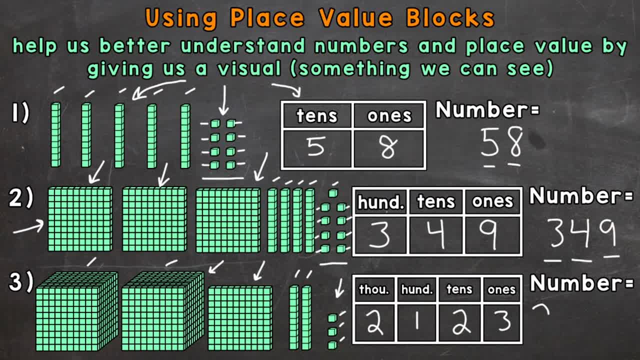 represent that. So our standard form would be 2123.. So the three represents three ones: two tens, which has a value of 20.. One group of 100, which has a value of 100. And then, lastly, two groups of 1000, which has a.